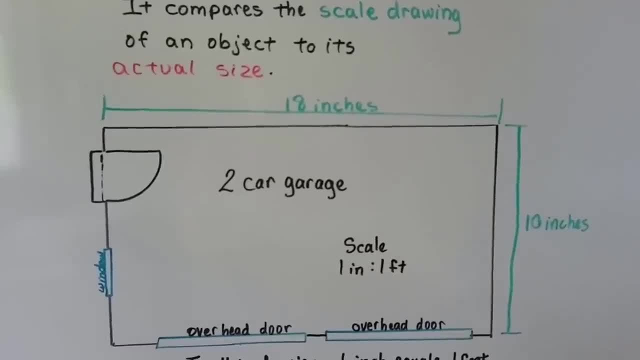 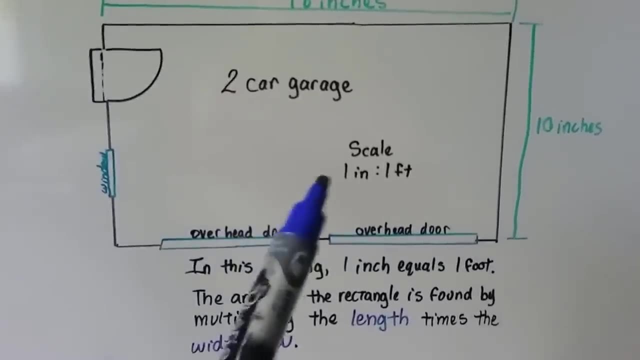 isn't really 18 inches by 10 inches. You wouldn't even be able to fit a toy car, hardly in that, would you. We've got a door here, We've got a window here And in this drawing, 1 inch. 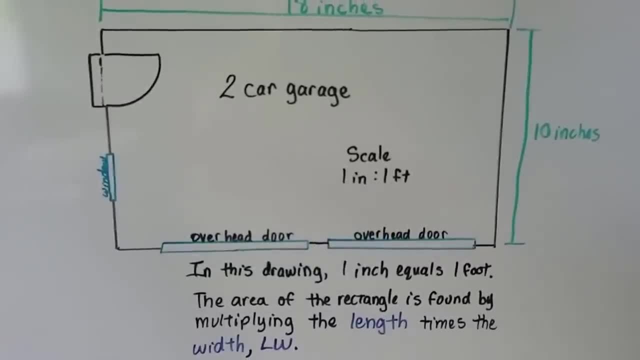 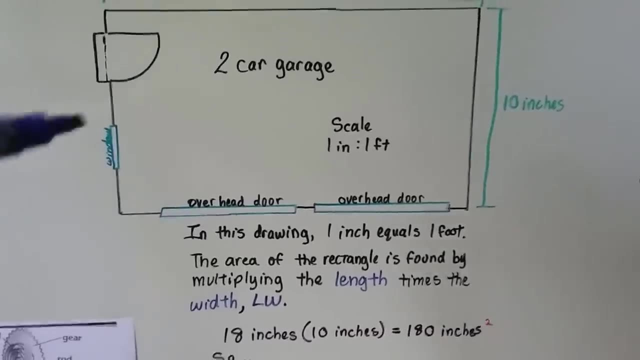 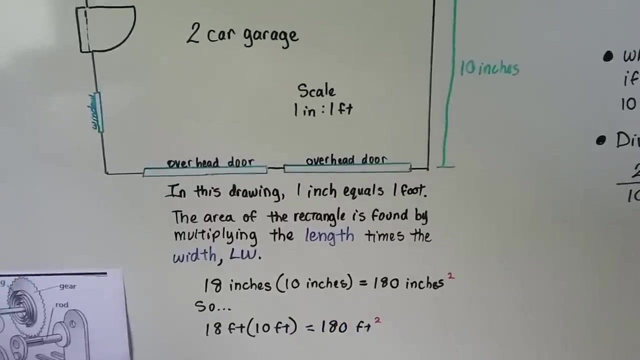 equals 1 foot, And the area of the rectangle is found by multiplying the length times the width, The length times the width. So we would do 18 times 10.. 18 inches times 10 inches is 180 inches squared, So that means 18 feet. 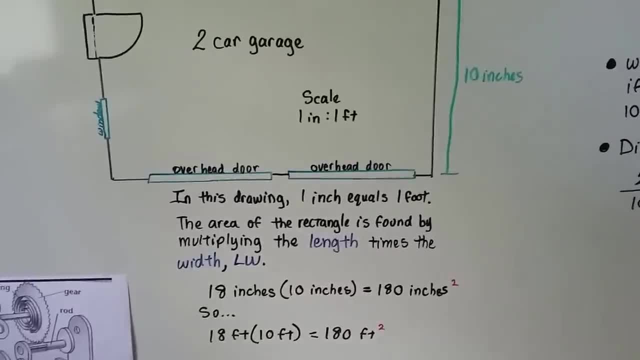 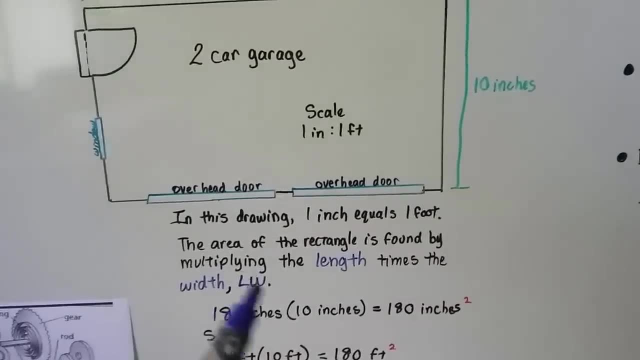 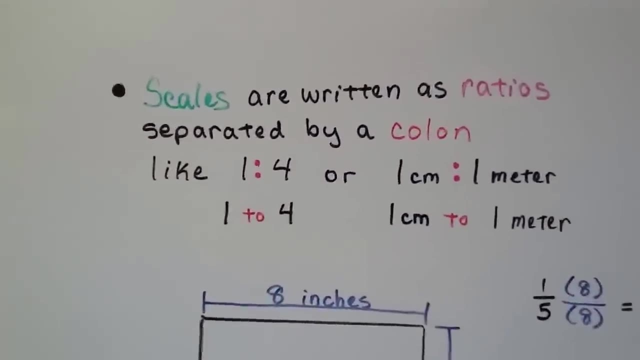 by 10 feet would be 180 feet squared, See, Because it's inches to feet. Alright, Remember, when you see the L and W next to each other, that means you're multiplying length times width. So scales are written as ratios separated by a colon. 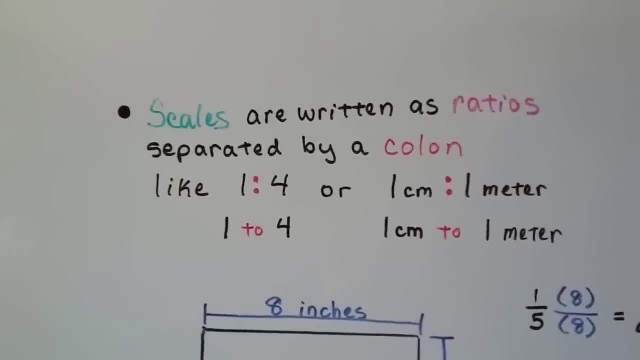 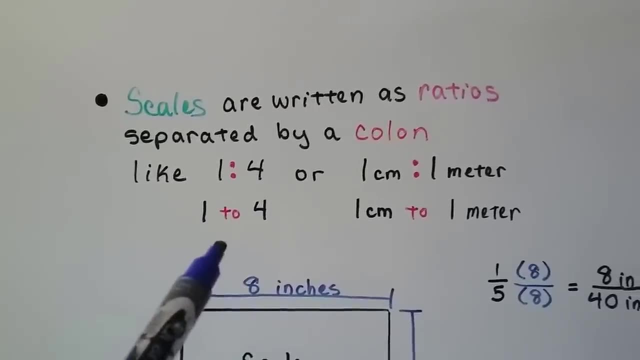 That's what these little two dots are, And it could be written as a 1 with the colon and the 4. And that means 1 to 4.. That's the ratio, Or it could be 1 centimeter to 1 meter. 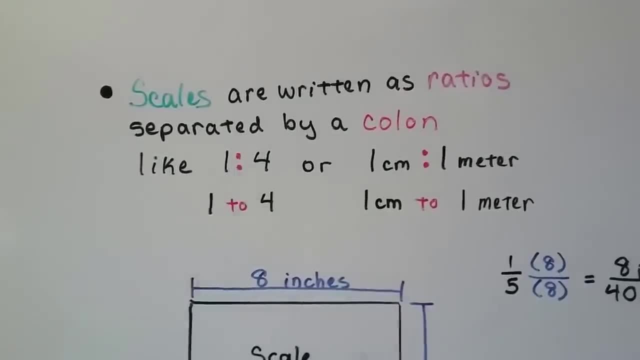 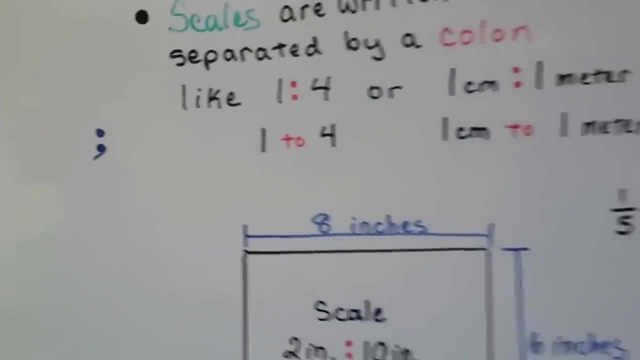 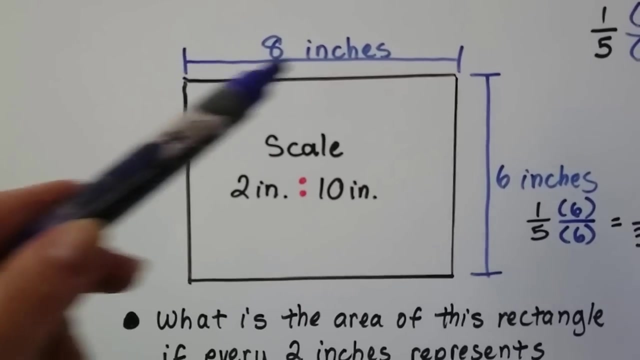 See, So these two little dots are a colon. If you see a dot with a comma, that's a semicolon. Alright, So a colon is just the two dots. So here we've got this scale drawing. It says this rectangle is 8 inches. 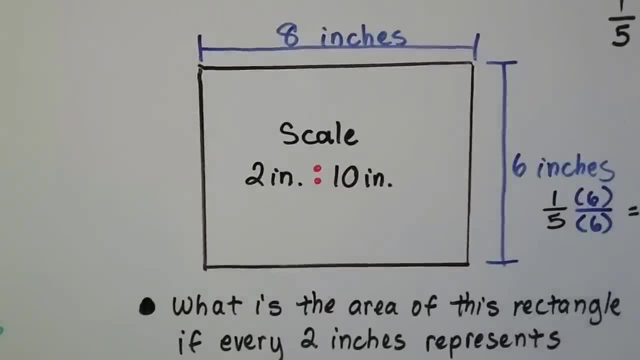 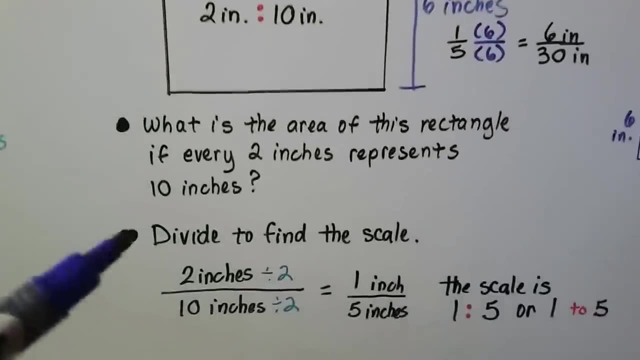 this way and 6 inches this way, and the scale is 2 inches to 10 inches. So what's the area of this rectangle if every 2 inches represents 10 inches? Well, we're going to divide to find the scale. We're going to write the 2. 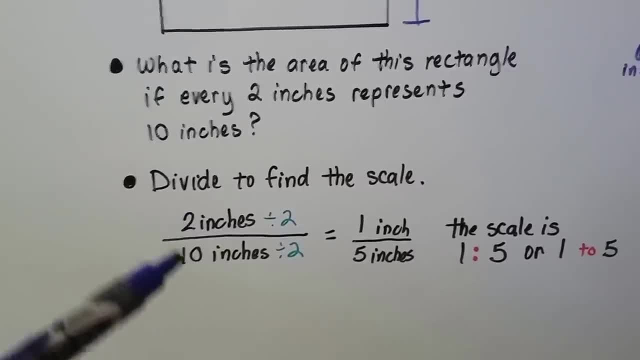 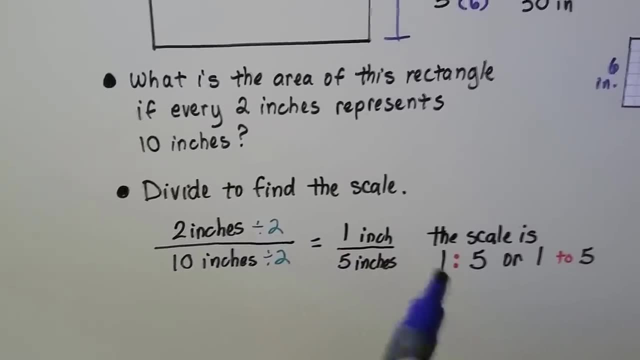 inches over the 10 inches, and this, as a fraction, can be simplified, can't it? We can reduce this. We divide both of them by 2 and we get 1 inch over 5 inches, So the scale is 1 to 5.. 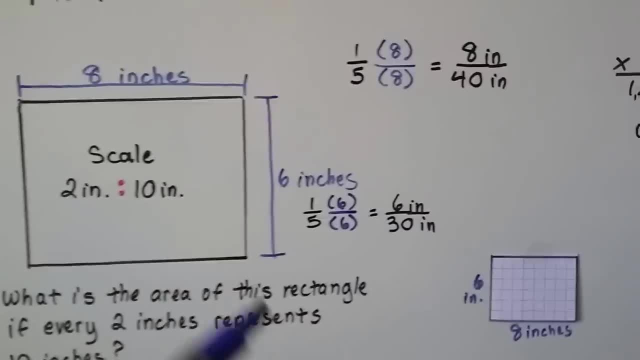 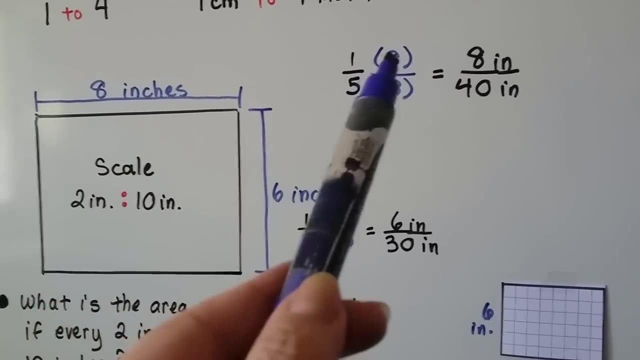 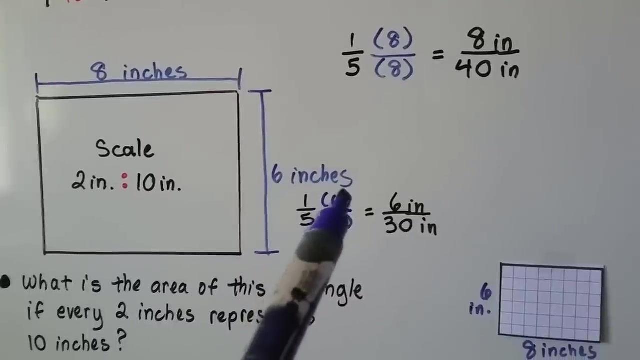 And what we do is we take that 1 fifth, that 1 to 5, and we multiply it, the numerator and denominator, by this 8 inches, And we get 8 inches over 40 inches. And we take the 1 fifth and we multiply the.